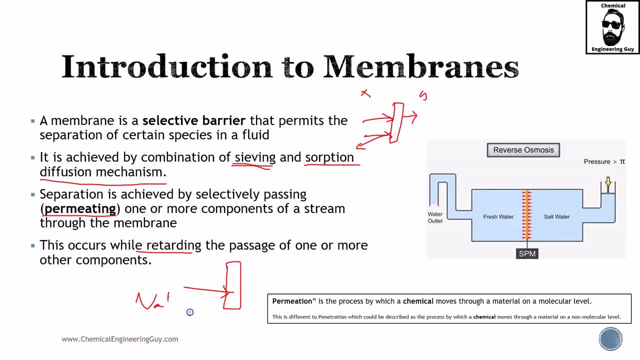 And so, like the sieving system I was telling you about, if you're focusing your attention in monovalent ions such as maybe sodium, magnesium, maybe chlorine, and you have a DNA strand which is, of course, huge compared to these molecules, well, the DNA will not feed through these pores. If we're 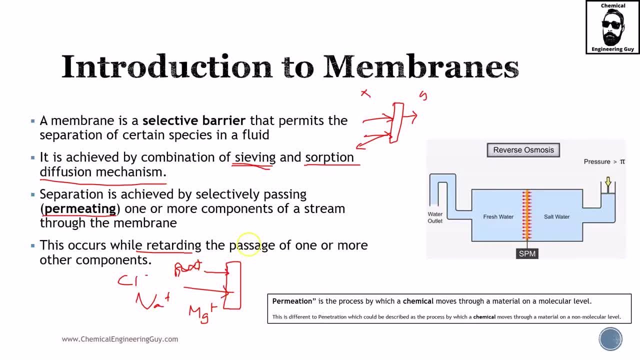 talking about pores of the size of one atom. DNA is lots of molecules, or let's say molecules bonded between each other. so retarding is not the concept right here. it's literally not passing through or not permeating an important guys to consider. maybe you have been studying mass. 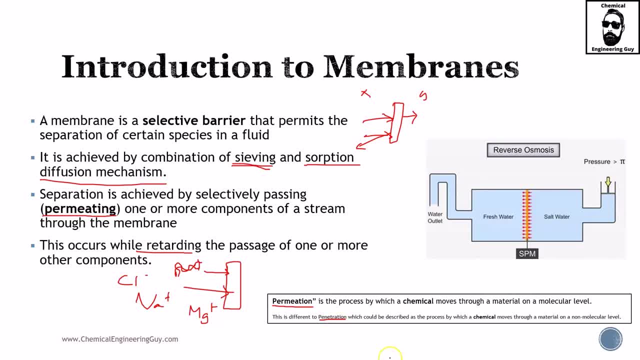 transfer already, so you know that penetration is also a important factor in mass transfer. let's define the difference. permeation is the process by which a chemical species moves through a material on the molecular level, which is different from penetration, which is or could be described at the process by. 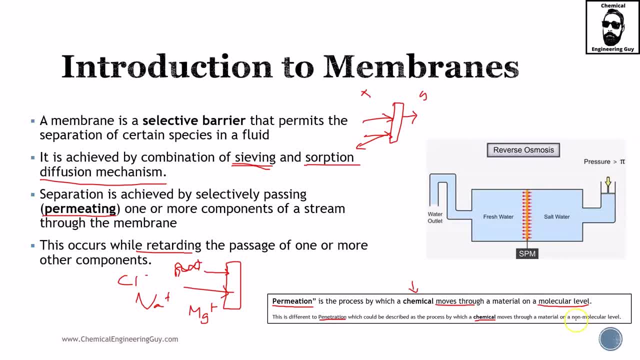 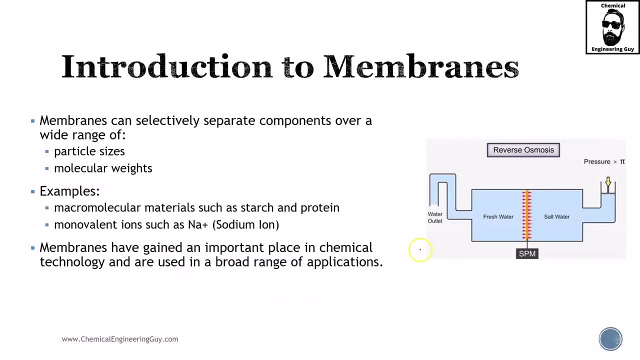 which a chemical species moves through a material on a non-molecular level. so that's interesting: one is at the molecular level and the other one is at the non-molecular level. okay, so membranes can selectively be separating molecules, and this can also beд is able to mutate a critical tissue into all these. 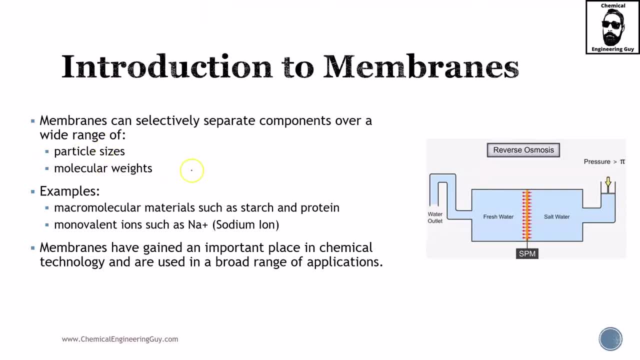 materials, depending on either particle size, molecular weight and maybe even charge. Examples are macromolecular materials. What do we mean with macromolecular? Maybe sugars, starch, proteins, nucleotides, the DNA, for instance? Or we can focus mostly into monovalent ions. 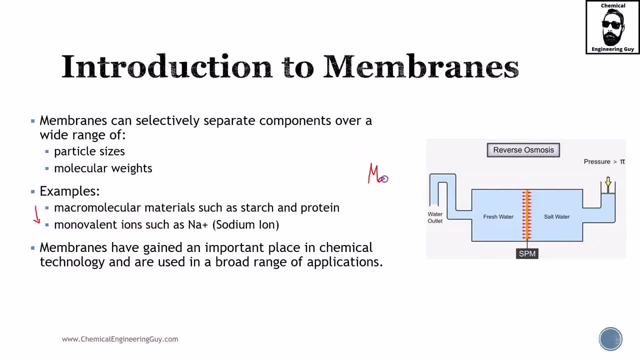 or let's say commonly, ions, maybe magnesium ion, maybe even the carbonate ion. There are many ways in which we could find ions which hopefully you get. the difference Macromolecular versus ions is huge, maybe a thousand or a million. I think a million is too much, but a thousand times. 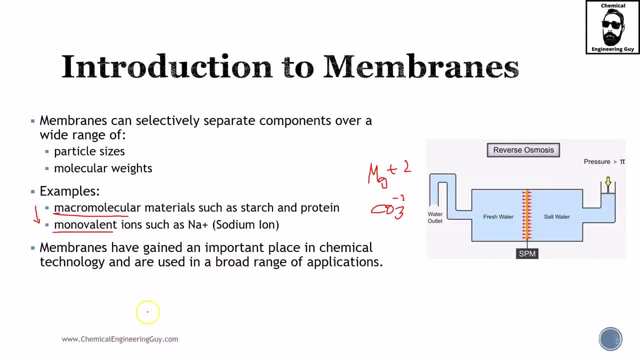 more is typically the case. Membranes have gained an important place in the chemical technology industry and are used in broad ranges of applications. Still, I would say that most of these applications are for water, but still we are getting more and more of them. 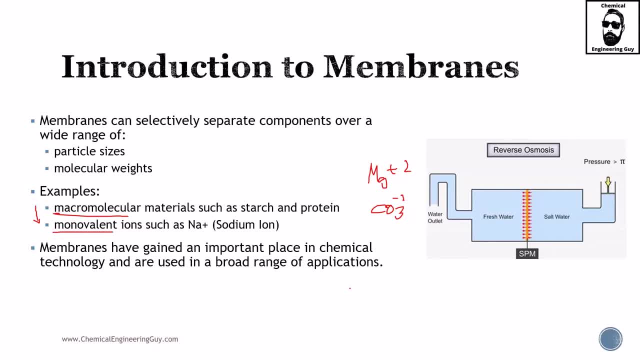 More applications. membranes are booming right now, not only because they are, let's say, seen as a novelty, but right now there are lots of material and when you have new materials you can test new type of membranes and see which type of interactions you get. Once again, the main: 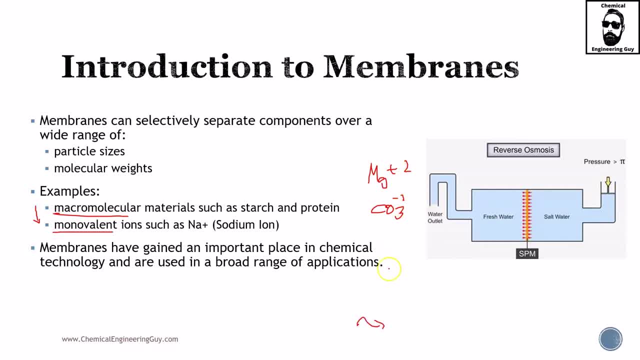 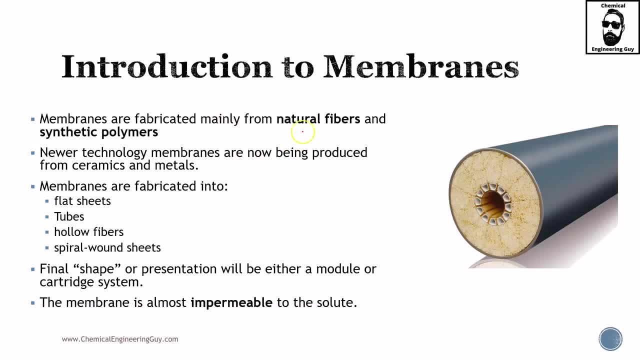 focus is in the molecular level. You want to see which and how the interactions are working within. Membranes are fabricated mainly from natural fibers or, more commonly, from synthetic polymers. Newer technologies- as stated before guys- are being now produced and new materials. 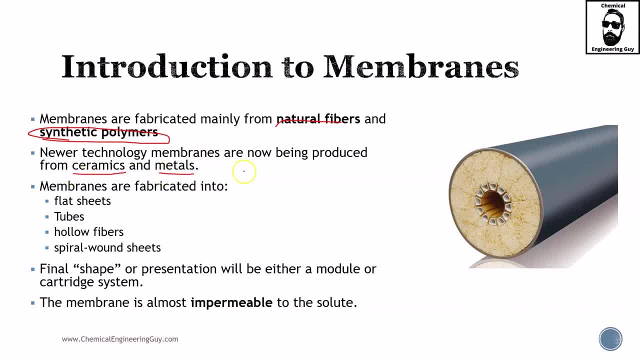 are coming into play, For instance, ceramics, metals or maybe, as stated before, natural fibers. We can think of the cellulite. Membranes are fabricated in different shapes. The most common ones: flat sheets, the normal filter. you will expect tubes, hollow fibers, which 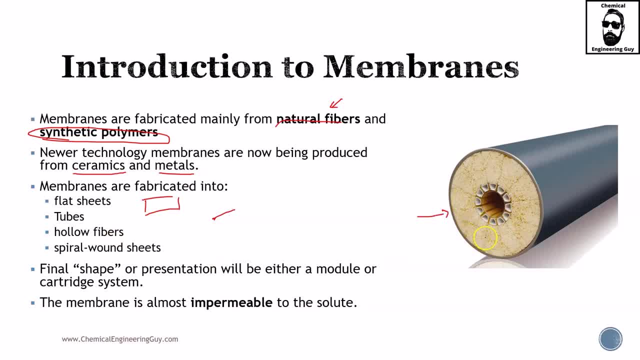 will be this example right here a little. let's say, one hollow fiber, Spiral wound sheets and so on. Now it's very important to consider that the final shape or presentation will be either a module or cartridge. This is the case here. As you can see, there are. 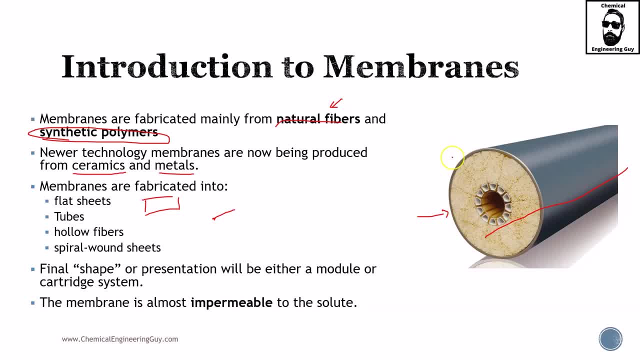 many hollow fibers. I don't know. I will guess thousand hollow fibers. Each one of them is carrying the process of membrane. So technically here we could say that we have million membranes happening at the time. but as engineering or engineers we will use a single unit. We will 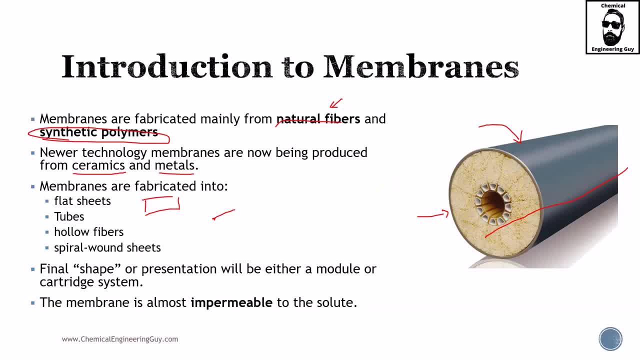 say this is the membrane system or the membrane unit operation, and we call this the cartridge system, which is also very common, especially in membrane technology. You will see that there are filters, cartridges or units instead of the actual unit per se, which is these hollow fibers. okay, 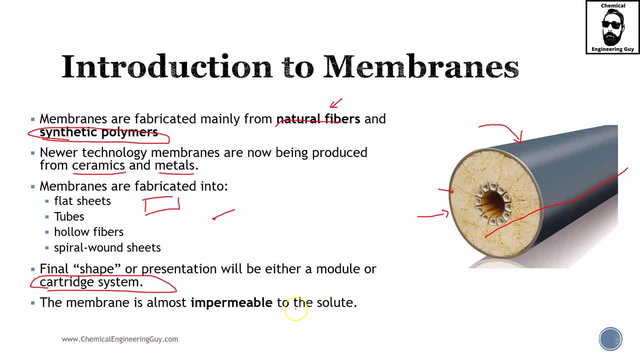 And finally, the membrane is almost impermeable to the solute, meaning that you want to avoid the certain solids which you don't want to separate and, of course, you want to see which materials will be separating. That's all the way, The main. 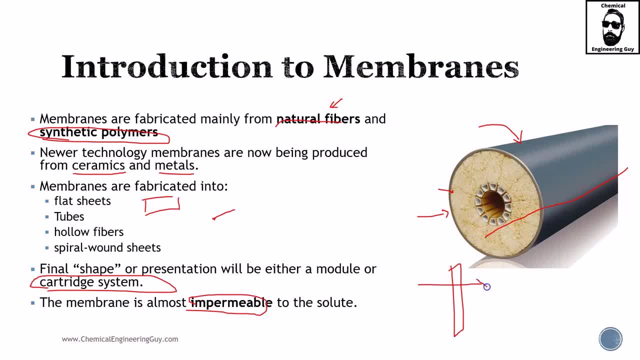 point of membranes is analyzing which molecules permeate and which molecules will not.